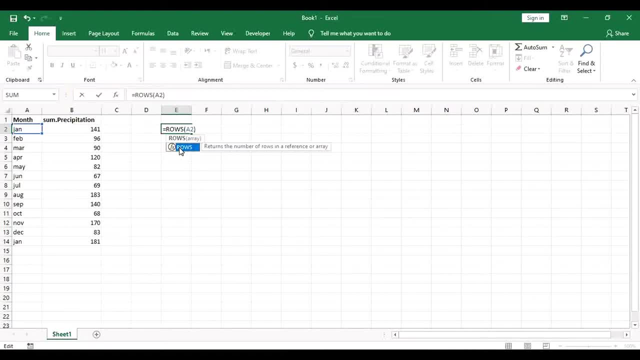 So don't make a mistake with this row function, because this one will count rows function. then it will tell you the number of the range you selected. okay, so I will go for this range and it will say it's 14 rows, as I can see here. so I said: 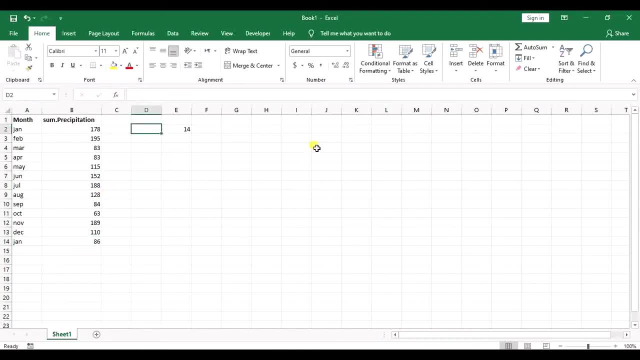 there are two ways, okay, so I will go for the first approach, and the second one is that I can just select the whole column that I want, to count the rows in it by going up the column and in this alphabetic character here, when the mouse sign appeared like this, I will select that. 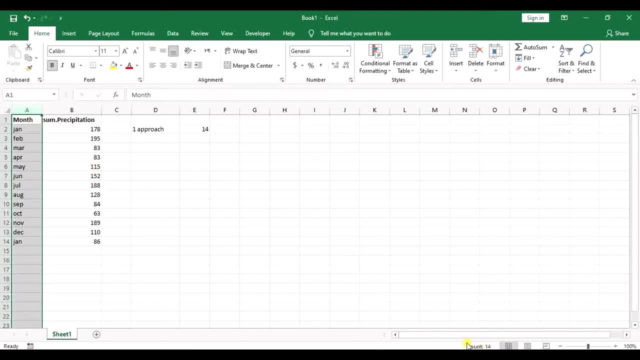 and it will just show me here. it will say: count is 14. okay, so I have 14 rows here and it says 14. so there are two tips for this approach. actually, this will just show you the number of rows that you have values in them. so 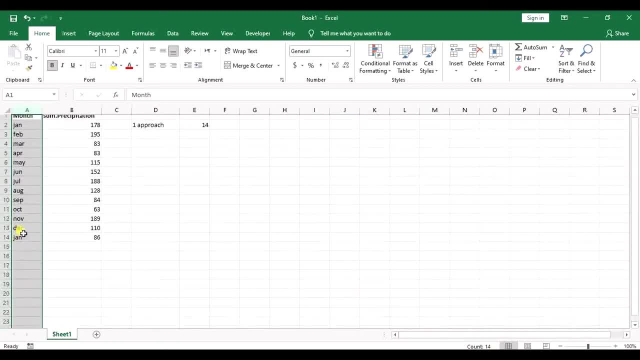 you can just select the number of rows that you have values in them. so you can select the number of rows that you have values in them, so you can just select. it doesn't count all these blank rows. and the other tip is that if I go here, 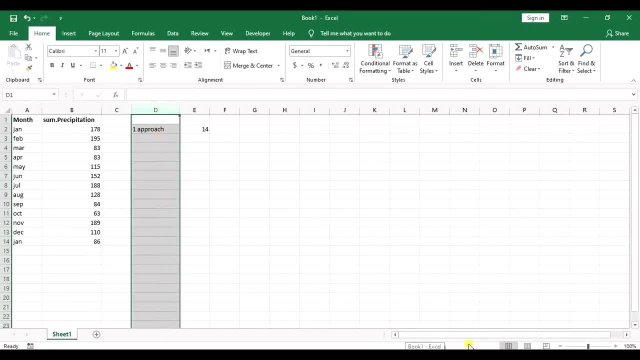 and select it, you can see there's nothing here, because Excel won't show anything. if you have just one cell of value in a whole column, okay, so it doesn't say it's one, it doesn't show it, it's blank in Excel site. okay, so I guess that's it for today's video. I hope you learned something new. 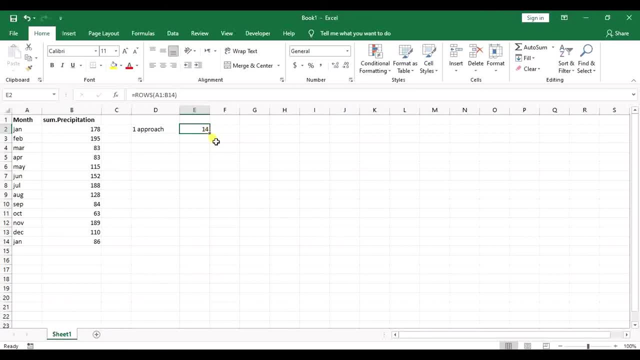 please don't forget to give this video a thumb up and subscribe to my channel. I will see you in the next video and bye.